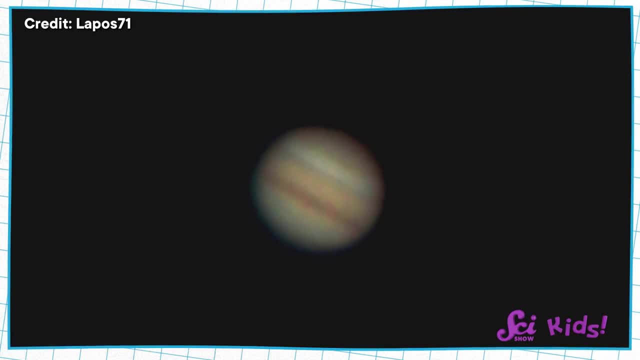 planets and other objects in space. Here's what Jupiter looks like through a simple telescope design. You're right, A simple telescope makes it a bit easier to see, But it's still not very clear in this picture. But what does it look like Telescopes? 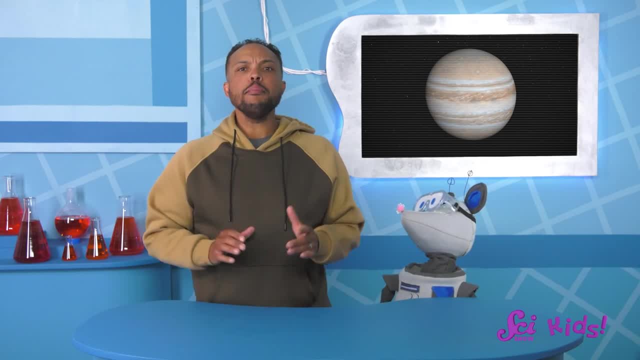 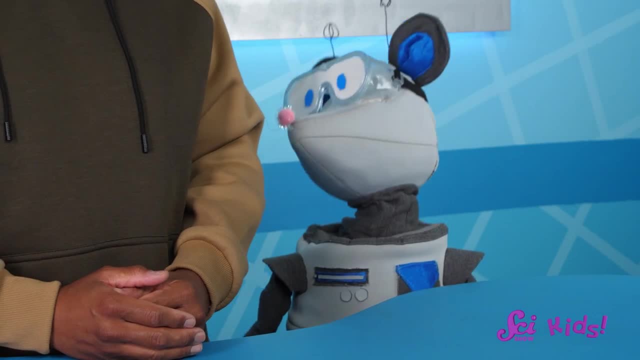 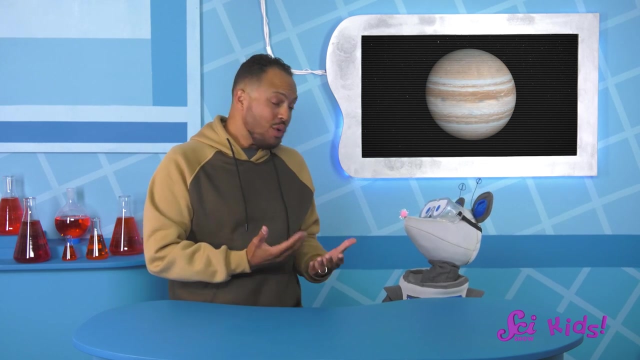 help us to look at things really far away. But if there's a lot of air between the telescope and the thing we're trying to see, it can be difficult to see. It can actually be hard to see through air. sometimes There's air all around us right now. 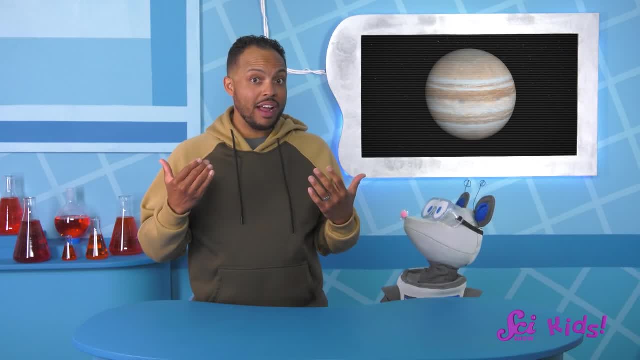 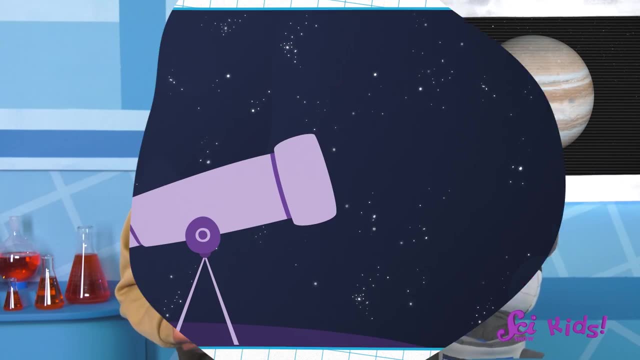 You and I can still see each other. so we think of air as being see-through, But it's not actually perfectly see-through. It makes the light that we see jiggle around. That doesn't matter most of the time, but a lot of air can make whatever we're trying. 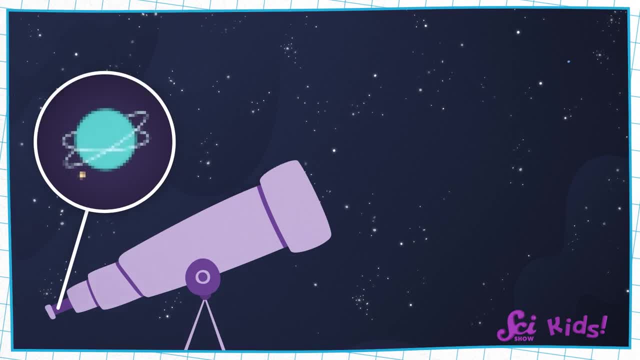 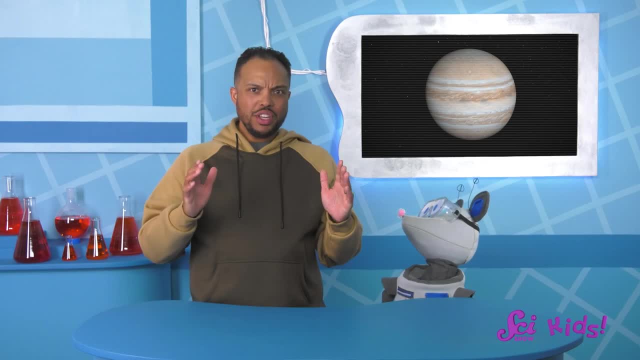 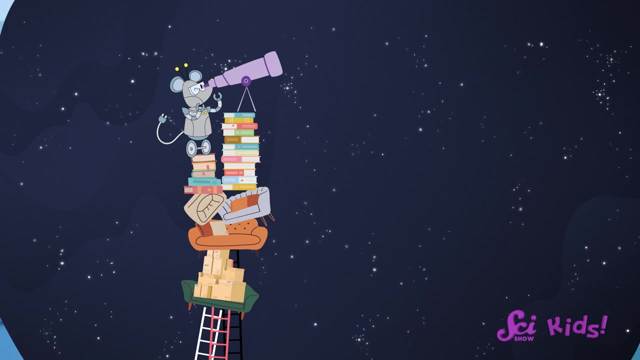 to observe through the telescope look blurry or fuzzy, So telescope engineers have had to come up with different solutions to make it so telescopes don't have to look through as much air. How would you solve this problem? Squeaks, That's a great idea. 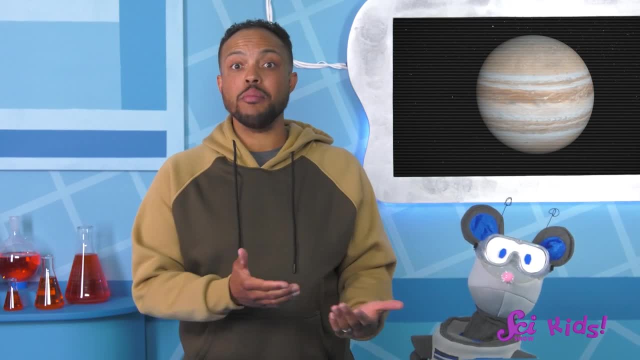 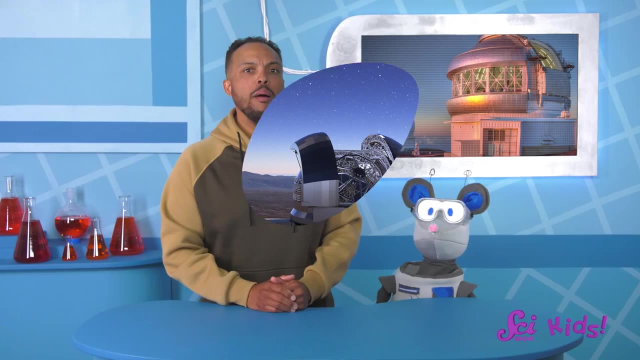 Engineers have tried a couple of different ways to put telescopes in places with less air, Like putting observatories in places that are really high up, like on mountains. That way the telescope is already closer to the stars and things up in space, and there's 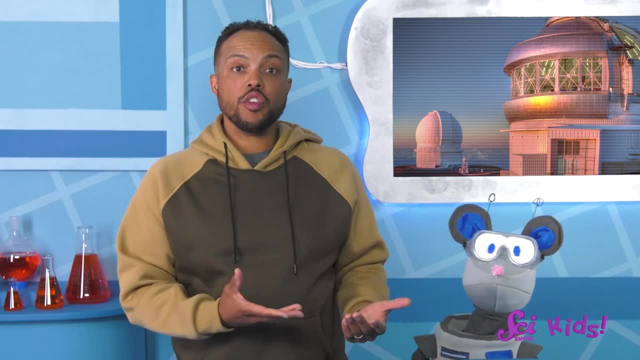 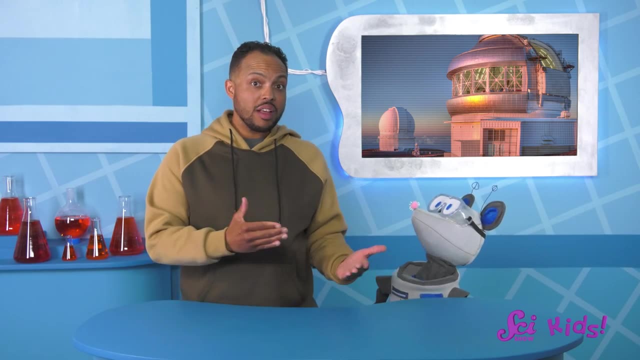 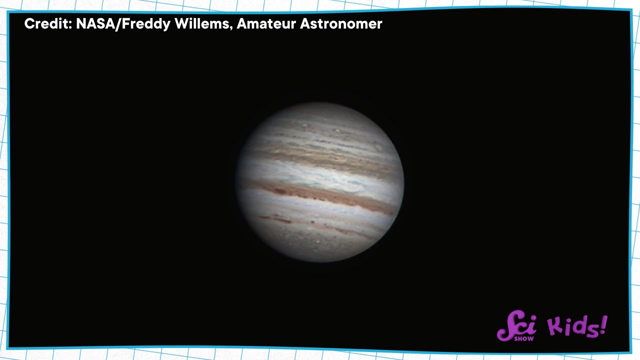 less air for the telescope to look through. People use these telescopes to see space really well while still staying on Earth. Yeah, we put Sam's telescope as high up as we could, so it works a bit more like this. Check out what Jupiter looks like from some of our high-up observatories. 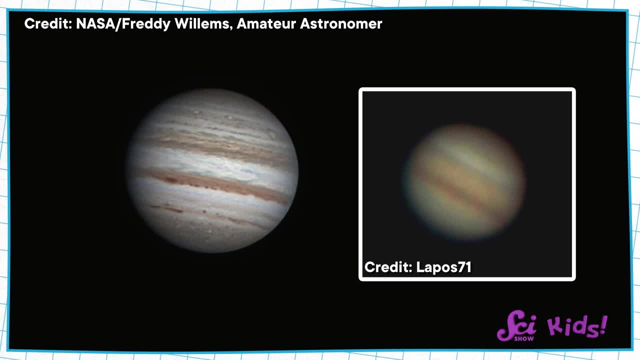 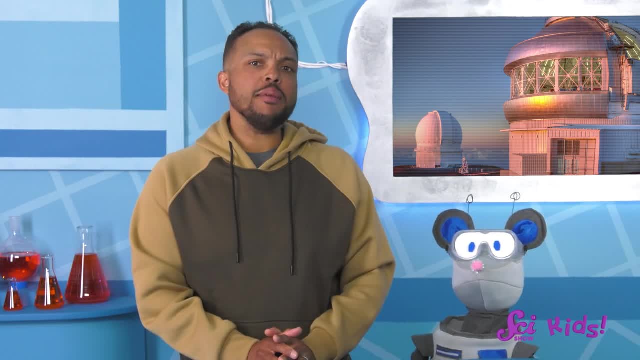 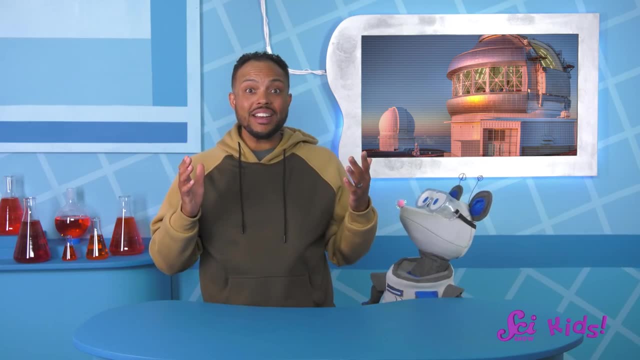 The photos are much clearer, But the telescopes are still on Earth, so some of Earth's air still gets in the way. So if we want to get a really clear image, we could design a different kind of telescope. Yes, we could design a telescope to work in space. 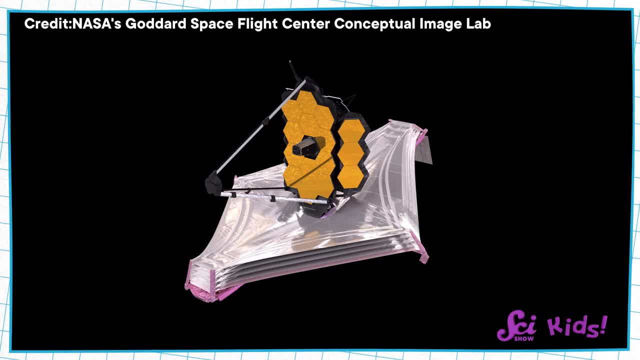 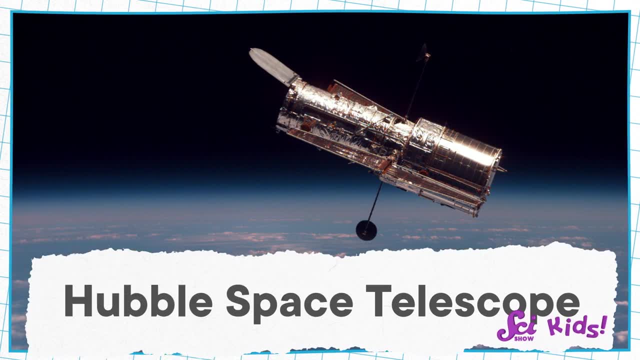 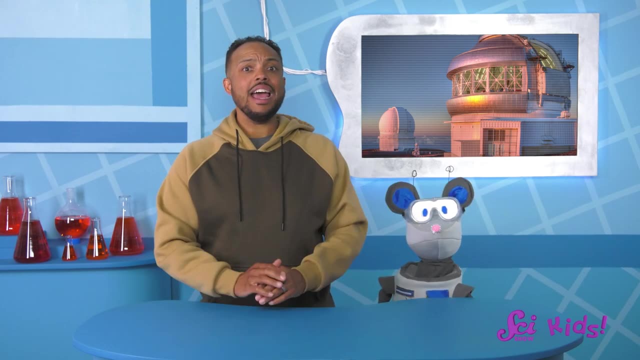 Space telescopes like the James Webb Space Telescope look really different compared to many telescopes here on Earth. They don't have the same kind of lenses and mirrors and they have to be much, much, much closer to the Earth. They're different designs. help these telescopes to look super far into space and then send. 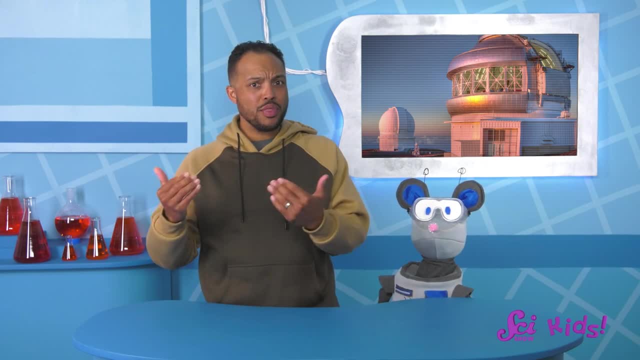 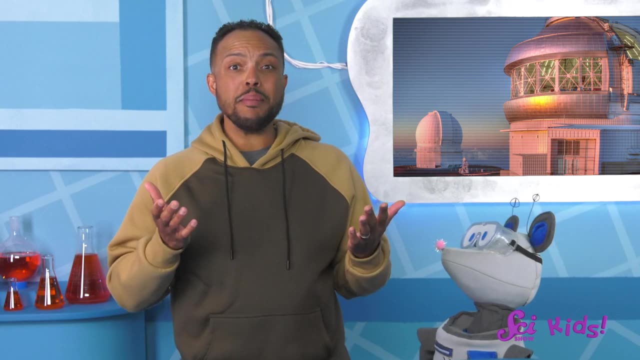 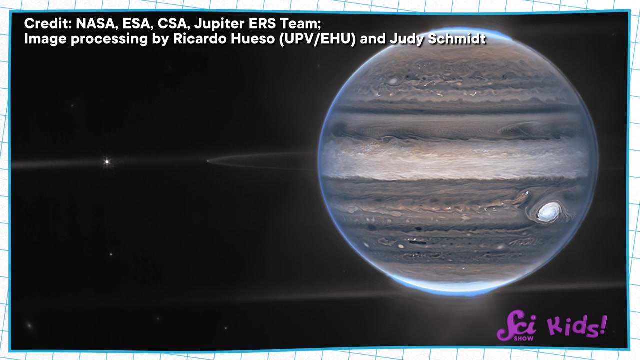 the images back to Earth. instead of having people looking through the telescope itself With no air in between the telescope and the things it's looking at, the images can be much clearer. Take a look. Sam sent me this picture of Jupiter from the James Webb Space Telescope. 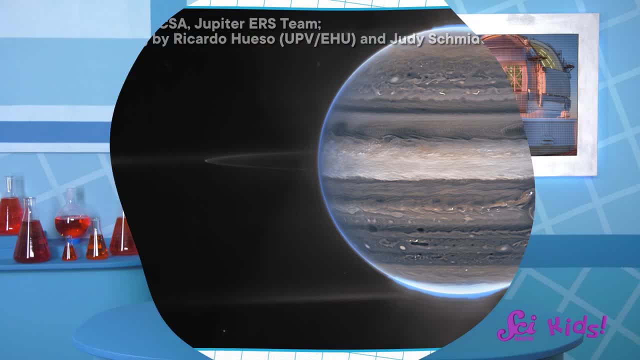 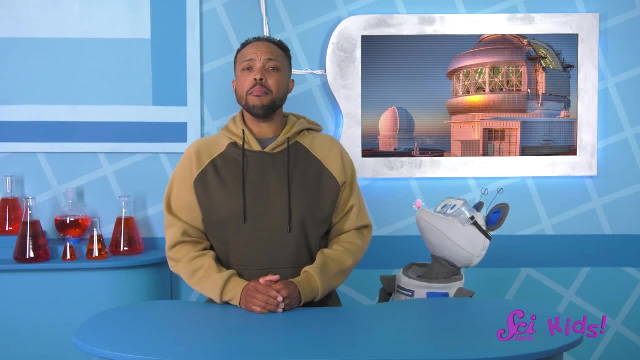 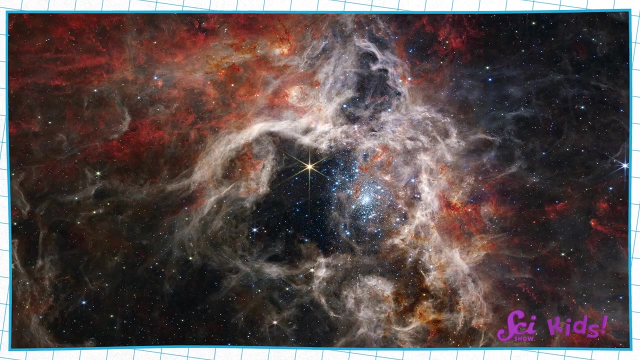 You can see the details of the planet so well, And we can even design telescopes to see things people can't. Some things in space can't be seen with our eyes, but they're still out there for us to learn about. We can design telescopes to see things we can't and show them in pictures. 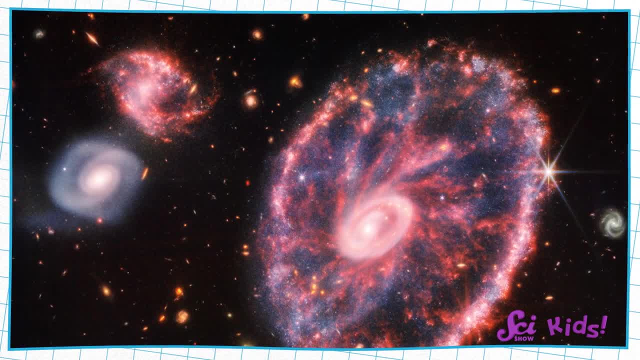 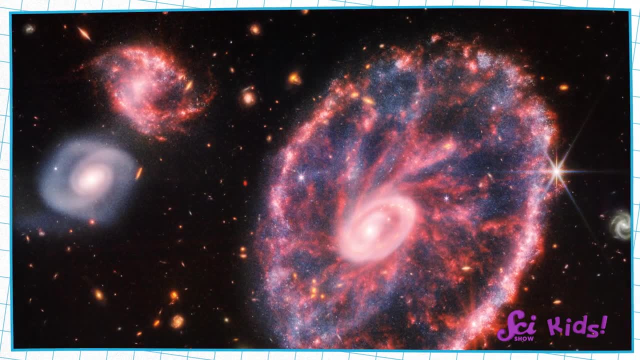 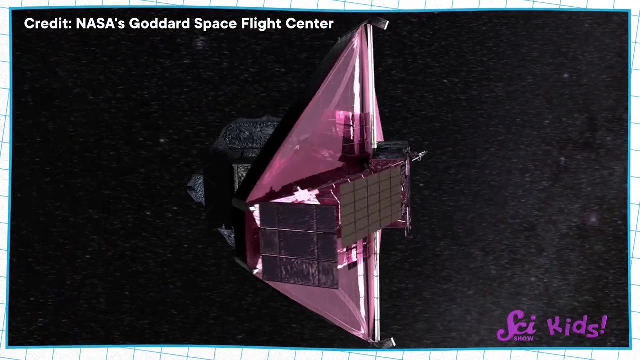 That means we can use the James Webb Space Telescope to observe space mysteries in amazing new ways and see whole galaxies like we've never seen before. This telescope took a long time and a lot of hard work to build And it's super far away from us now, so designing it to do lots of important observation. 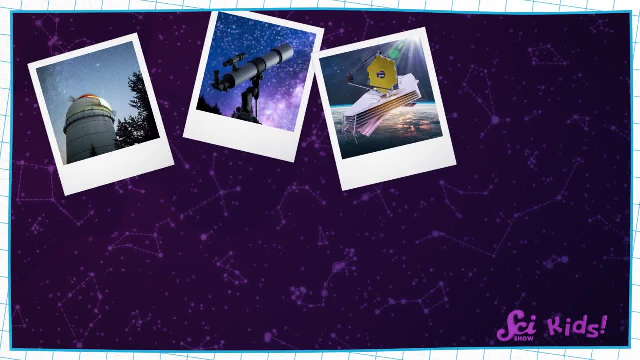 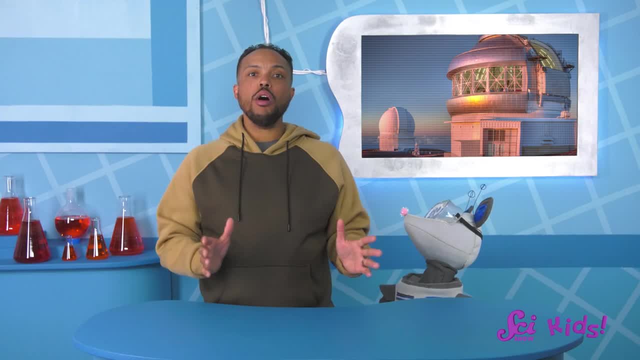 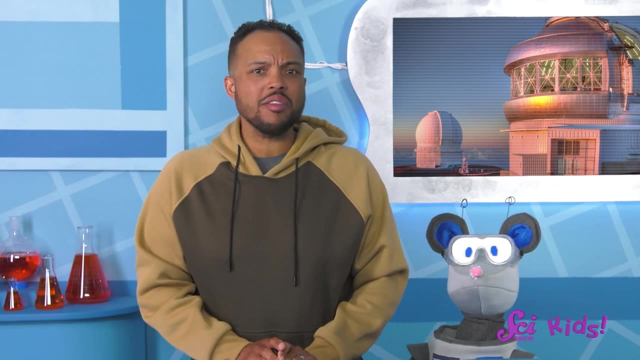 jobs well was really important. Telescopes come in many shapes, sizes and even locations, and each design can be used for a different purpose. Our small telescope is great for playing and observing stars at home. Sam the Bat's telescope is great for his special space observations. 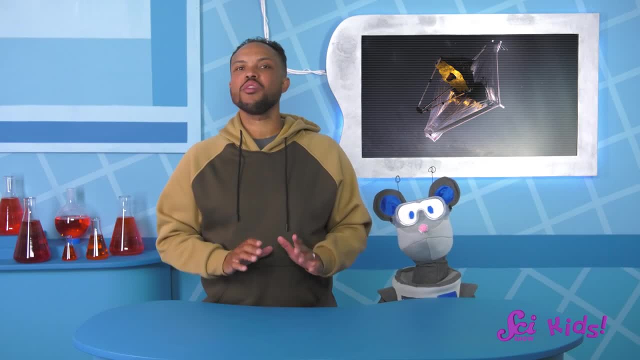 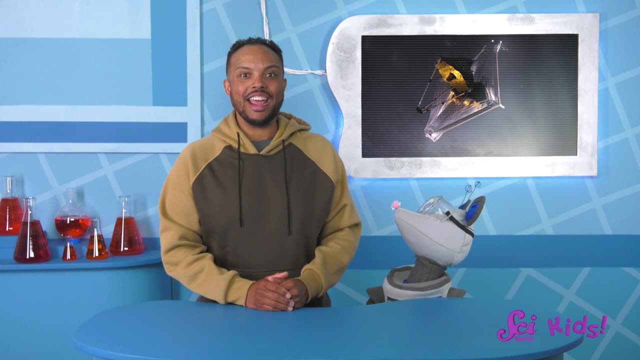 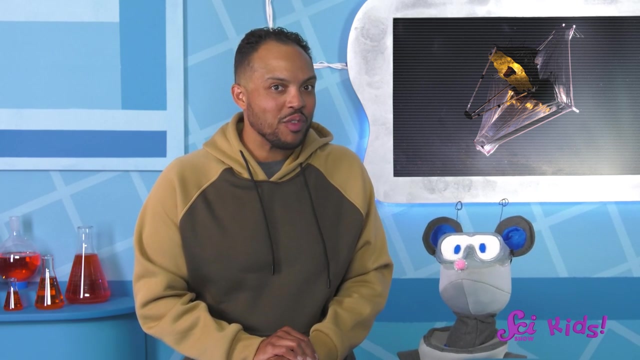 And the James Webb Space Telescope is going to help us make discoveries no human has ever seen before. I bet that Sam will be really excited to answer your new questions about the James Webb Space Telescope Squeaks. But speaking of questions, how about we answer a quick question from a viewer first? 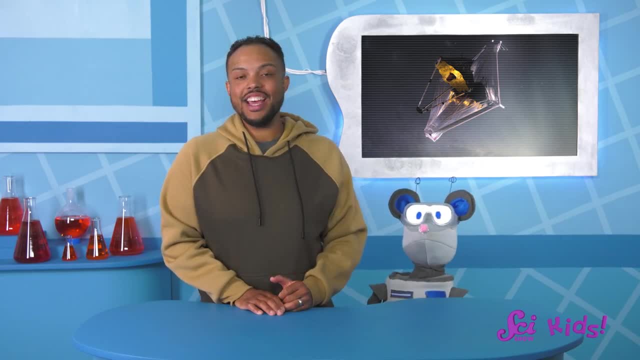 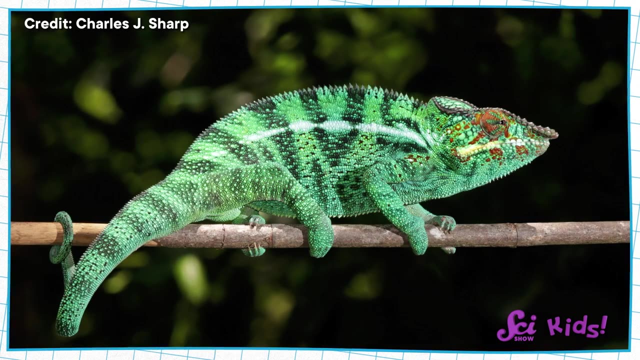 Today's question comes from Vibha, age 10.. Vibha asks: How does a chameleon change colors? Panther, chameleons are amazing lizards that can change the color of their skin from green and blue to yellow and orange, white and red. 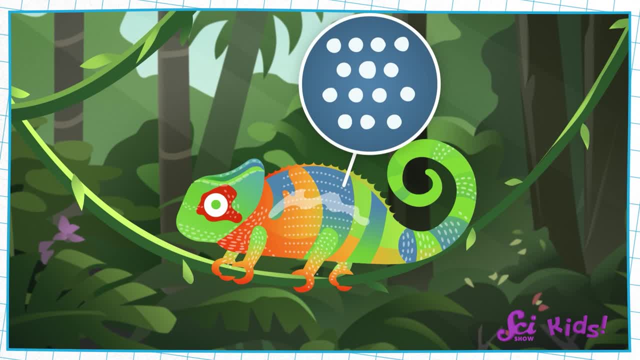 A chameleon's skin is filled with lots of teeny tiny crystals called iridophores. The iridophores have a special structure or shape that makes the chameleon look a certain color when light bounces off the crystals into our eyes.